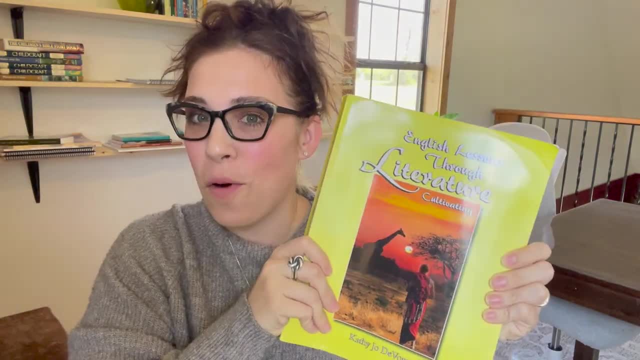 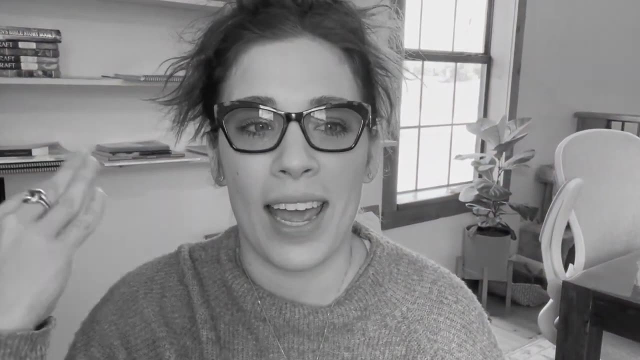 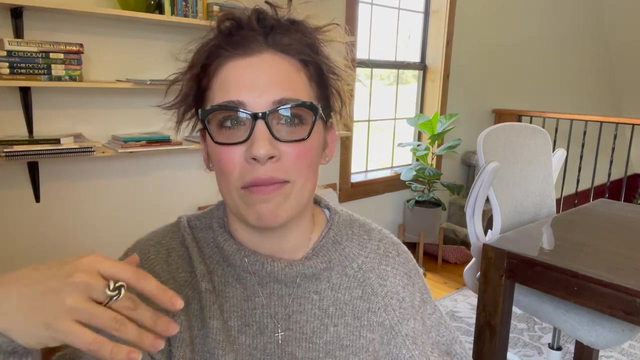 selected English lessons through literature for my fifth grader, as well as my- no, no, no. fourth grader and my sixth grader. I've been making so many of the next year videos. I'm now saying they're upcoming school grade. I apologize. So fourth grade and sixth grade, The book that I 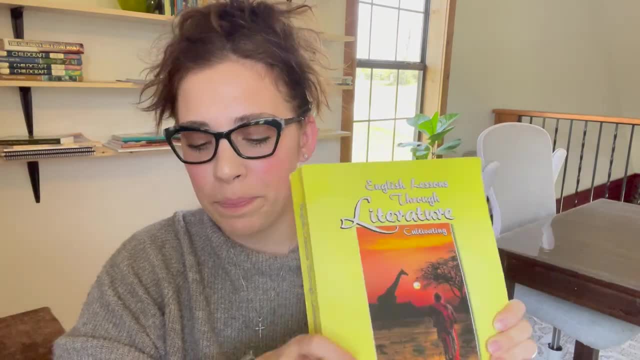 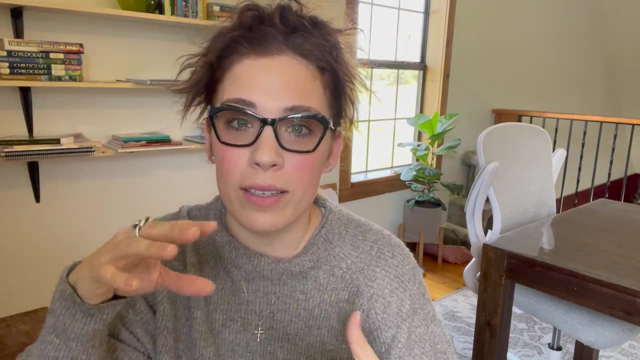 am holding here today is going to be my fourth grader's book. What we're going to discuss today is really how it works, where I bought it, some tips, hindsight things like that that you can use to help you with your writing. So let's get started. 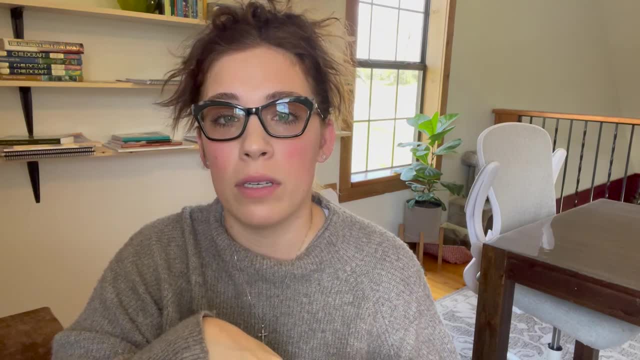 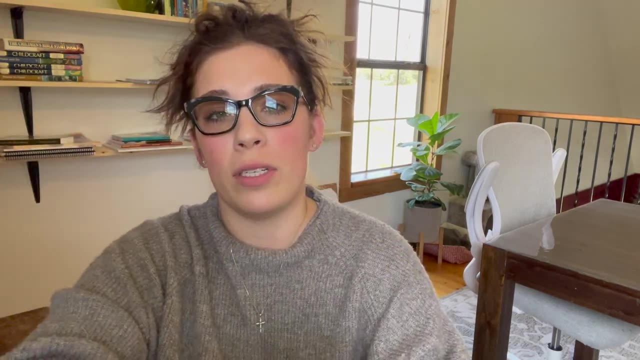 So what you can do to be prepared when the book comes in the mail if you choose to use this program for your student. So, English lessons through literature. I purchased it through Rainbow Resource. It is a literature-based program, So if you are finding that some of 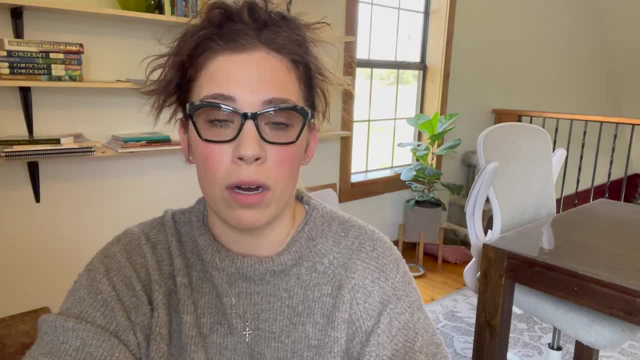 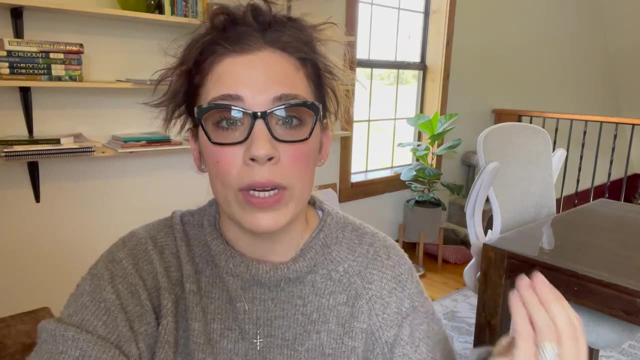 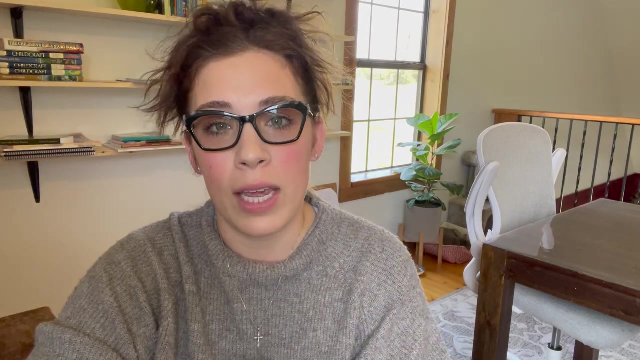 the language arts programs your students are currently using in the home or have used in the past are very lengthy and there's just a lot more additional readings that's assigned to it. this, the readings, are a part, are part, of the actual curriculum itself. So they will read a. 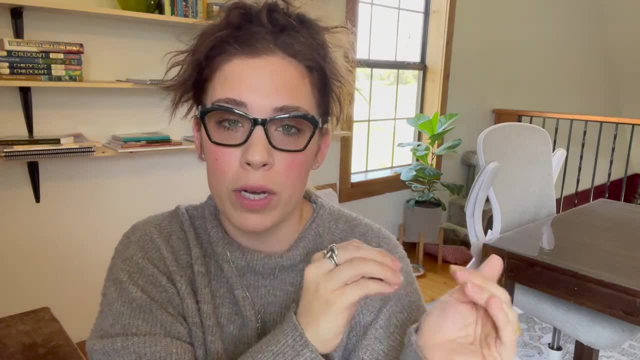 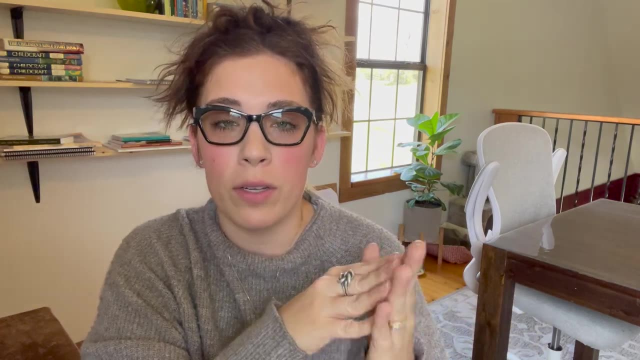 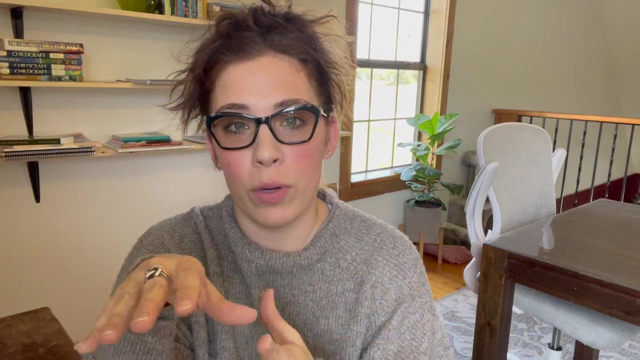 passage they will be reading parts of shorter story books or fables. They're typically available through public domain or you can get the books at libraries, So it's not going to be anything new or something that you can't really obtain. Then the student is going to walk through the 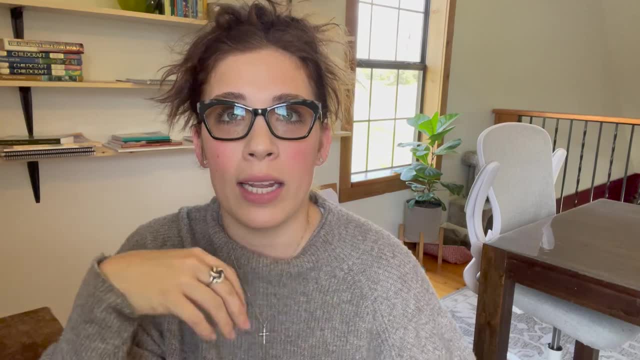 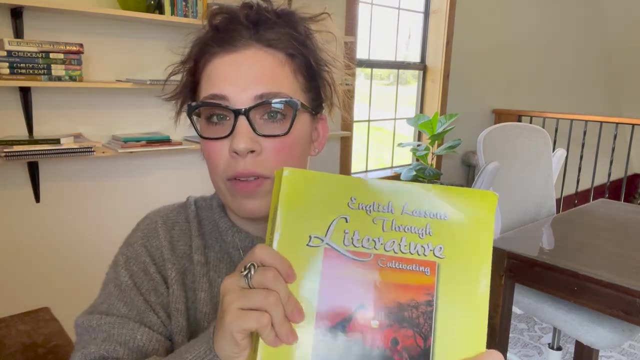 stories that they, that they had just read. And let's say they're being asked to read a book and they're going to be reading a book and they're going to be reading a book and they're going to be introduced to what a noun is They will use in this book. they use part of the story that the 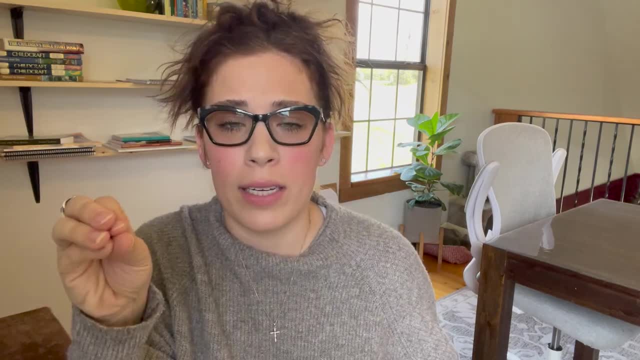 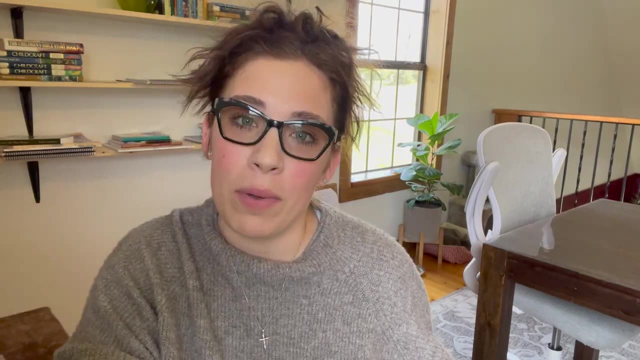 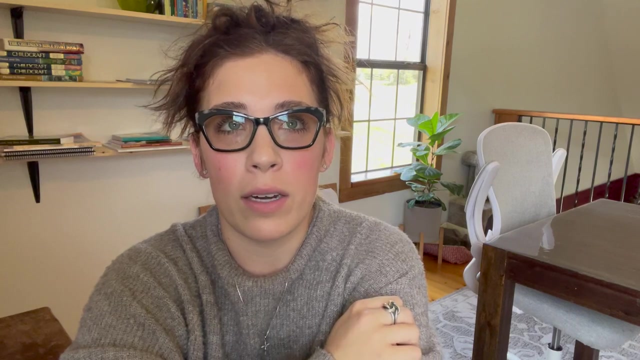 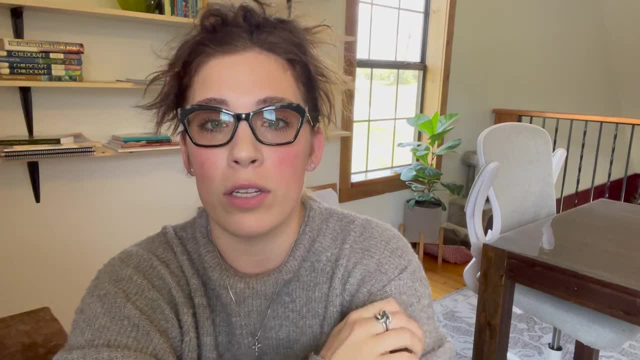 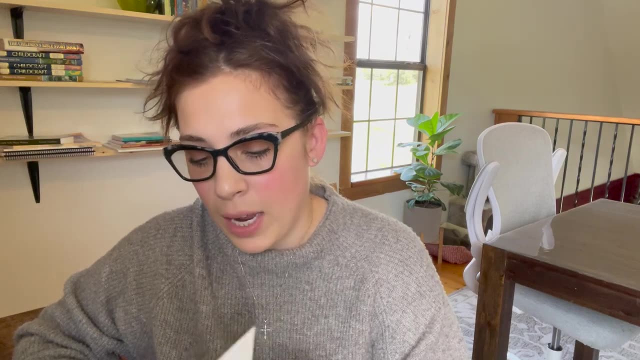 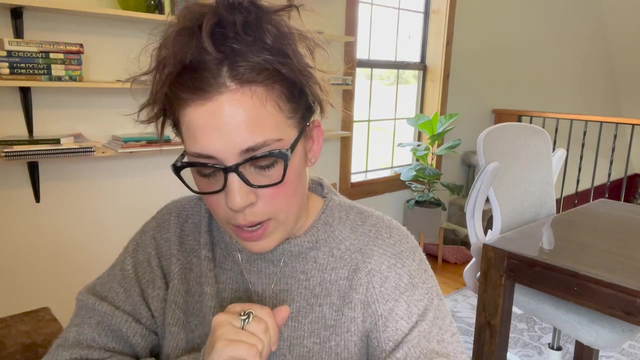 you can read it in black and white, So you could. if you really wanted to see the full color version. there are instructions to do so in the book itself and where to find them. everything isn't in the very beginning of the book. Sentence diagramming- that's introduced in here as well. 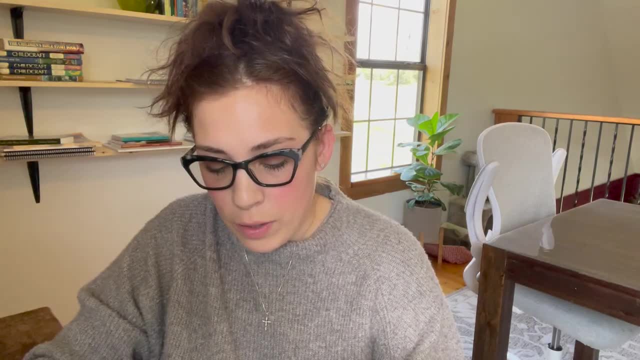 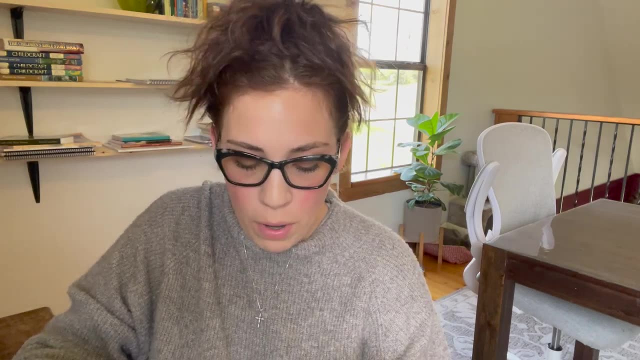 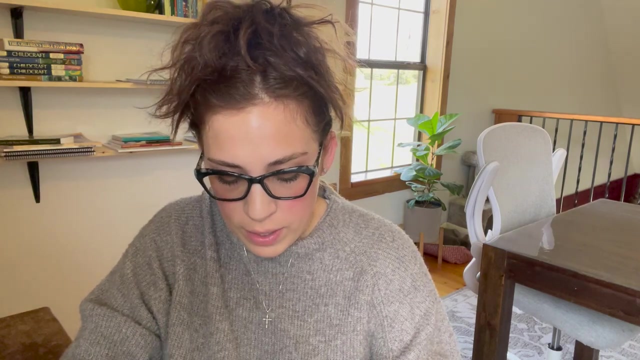 I'm just taking a short look to see if I'm missing anything. They also get to play with sentences, so they'll be presented with the sentence and for example, it says: change the nouns, Change proper to type, so declarative, interrogative, things like that, changing adjectives and then 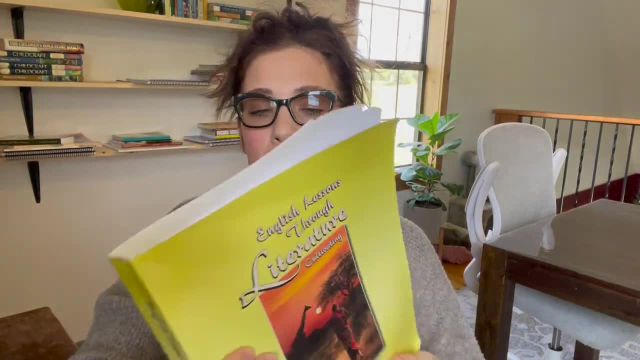 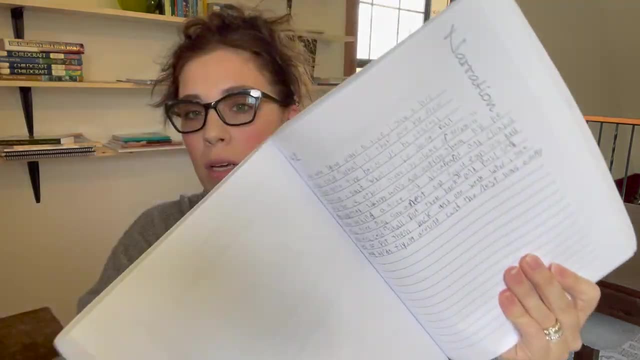 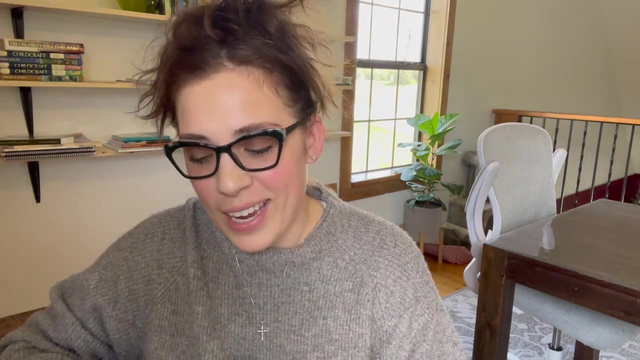 there's in the exercise workbook here. this is where they're going to actually be doing all of their work. so there's copy work that your student will be going through. everything that you will see in a traditional language arts program- Charlotte Mason style you will see in here. this program worked so well. 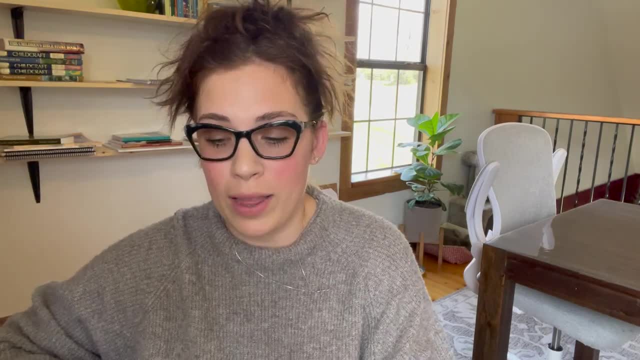 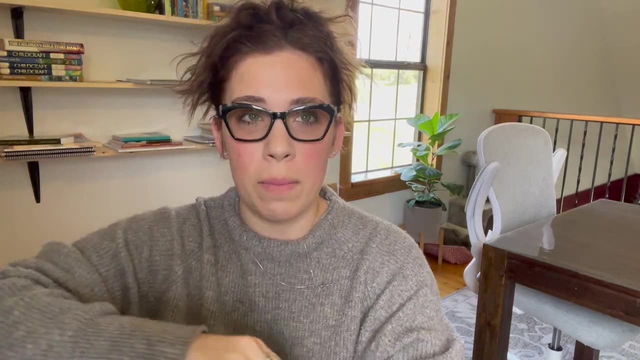 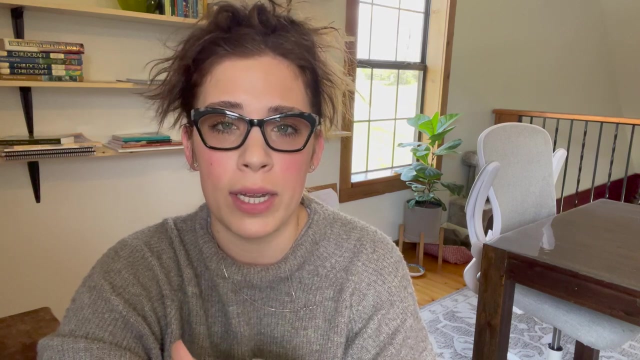 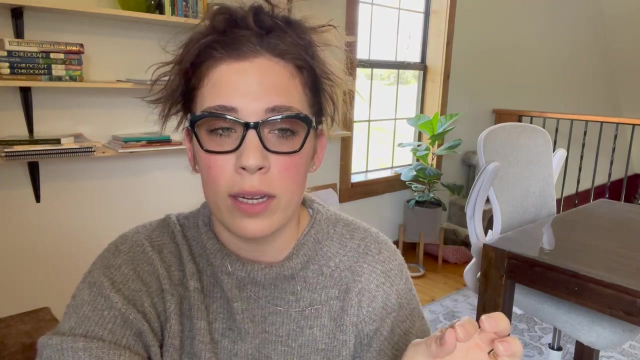 for my son. I love this program. I love being able to just sit and read with my son and I felt like it was very easy to follow. it typically took him including reading his chapter for the. the exercises that was presented to him, I would say 20 to 30 minutes at the most. exercises are short. they are in my 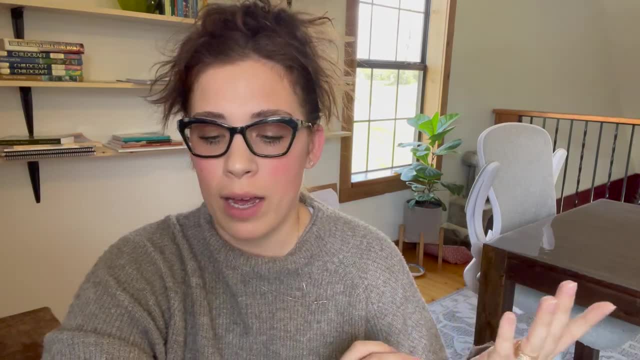 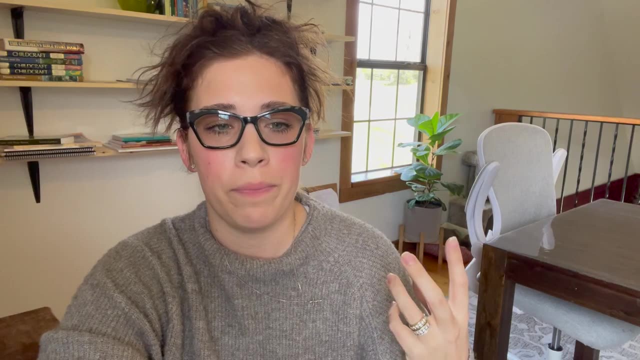 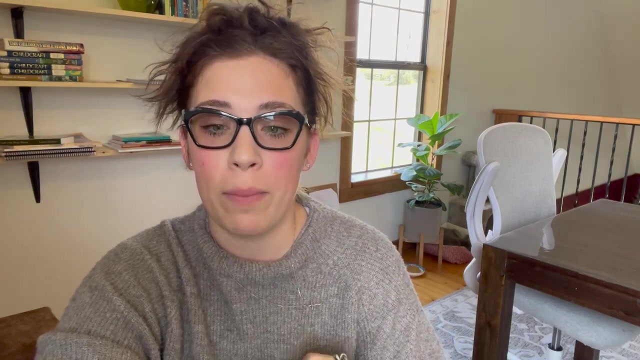 opinion, easy to follow and learning to understand. they require a very structured and including a degree to understand a Europe is available both, so if you or students really need the training, that's part of your program in a traditional manner. so this seems like one that should have been addressed, but 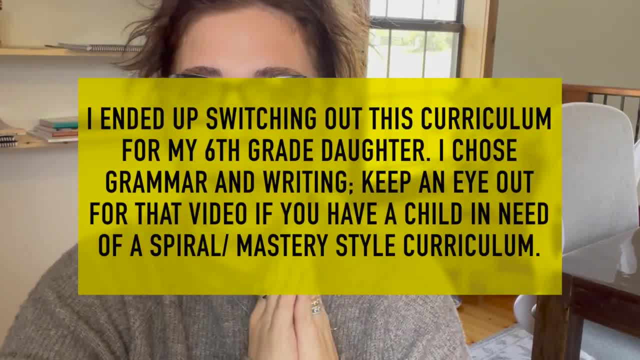 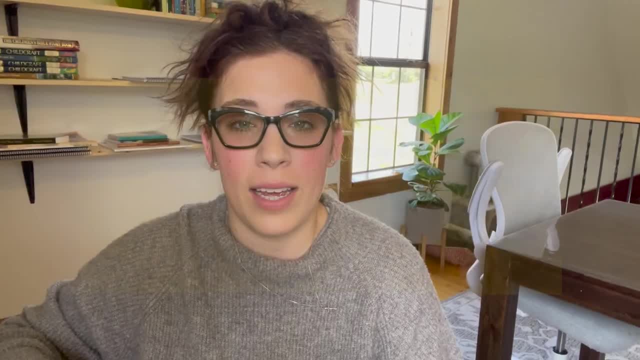 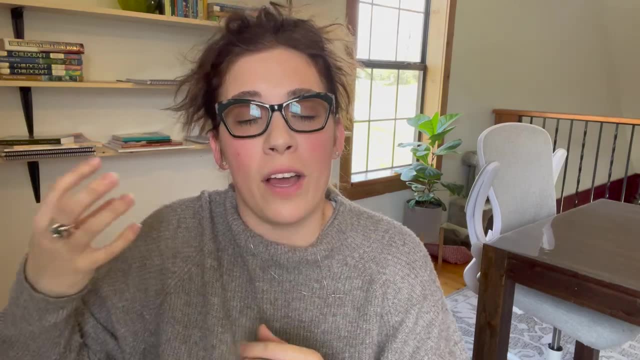 is something that that that helps your students, so it is something that is something that is outstandingly cool- when you know is there is no extra wording that made it confusing for a student to comprehend, or at least grasp- is interwoven into literature And I think for her, the idea and the concept of what 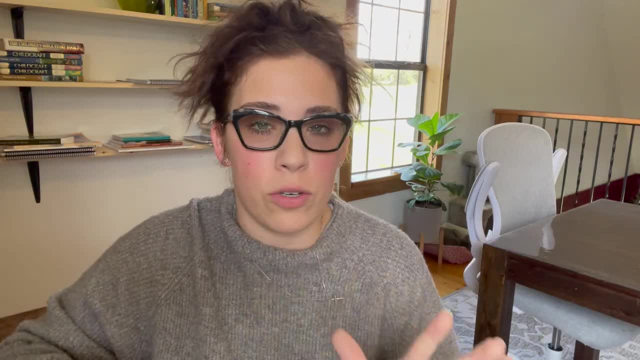 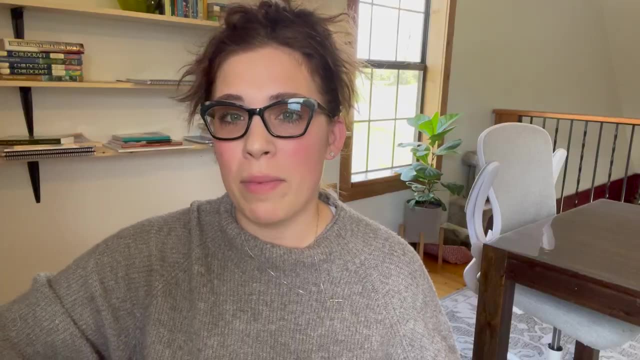 she was learning for a sixth grader. it was just kind of lost in the translation and then she was captivated by the stories that she was reading. I hope all of that makes sense. Let's talk about some of the things that I did to make this program smooth as butter. 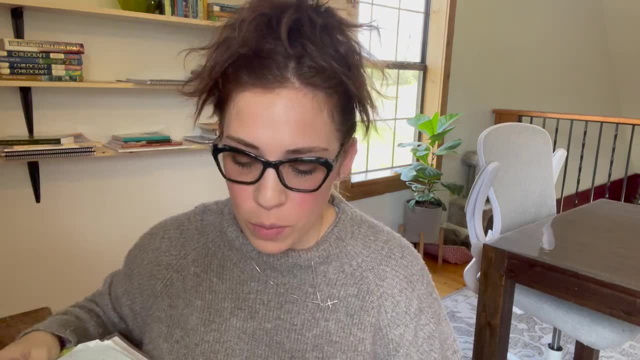 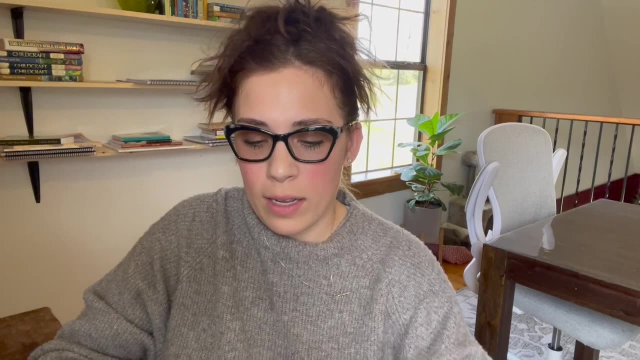 So in the back of the student workbook- it's either going to be the student workbook or the actual lesson plan book itself- There's an appendix and I went ahead and just copied it off because I didn't want to rip it out and then mess up ripping it. So there's an. 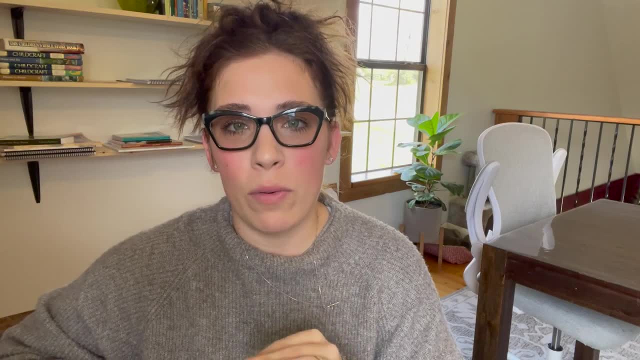 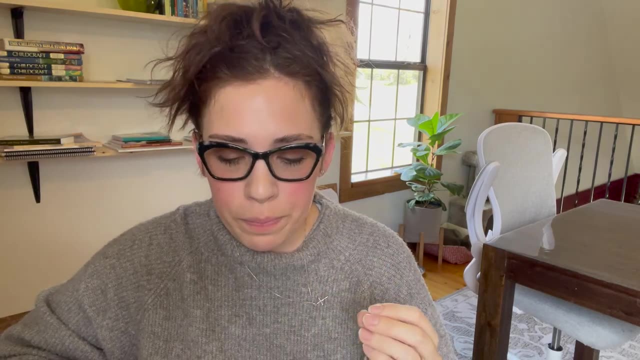 appendix in the back that your student every day will read part of the appendix, depending on what grade they're in. it'll tell them in the book And this is memory work. So this is where your student is going to go through and I'm just going to look at it and they 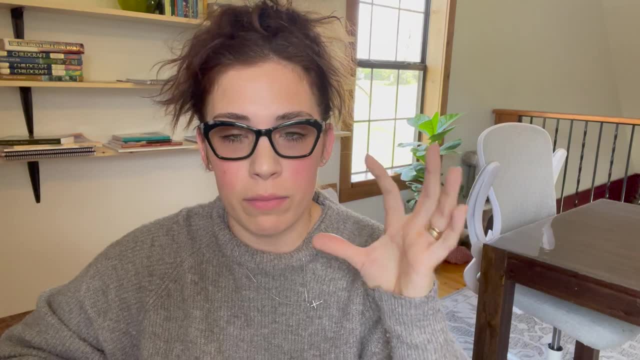 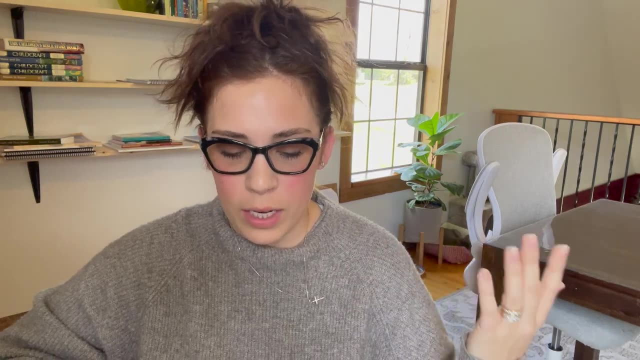 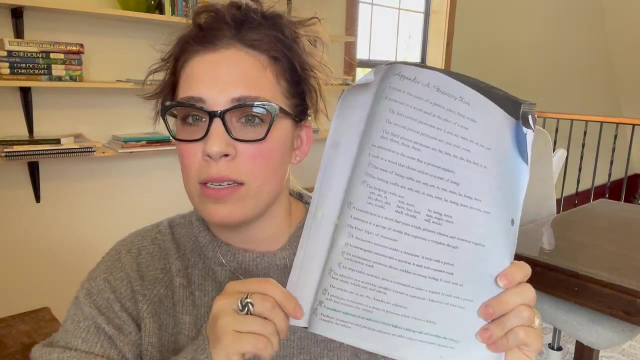 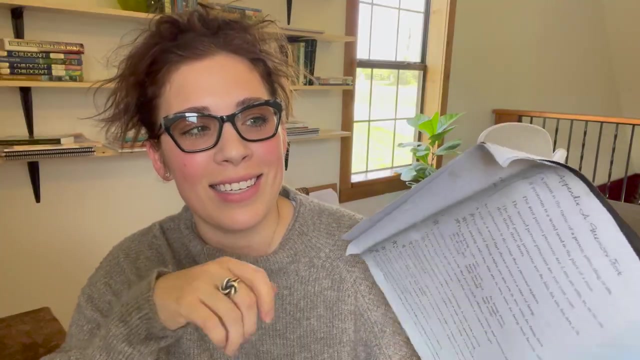 are going to recite you their section in the appendix every day. a noun is a pronoun, is a verb, is a conjunction, is, and they're going to go through and they're going to recite this to you. I would recommend just making a photocopy of it or, if you're more brave than myself, rip it out and staple. 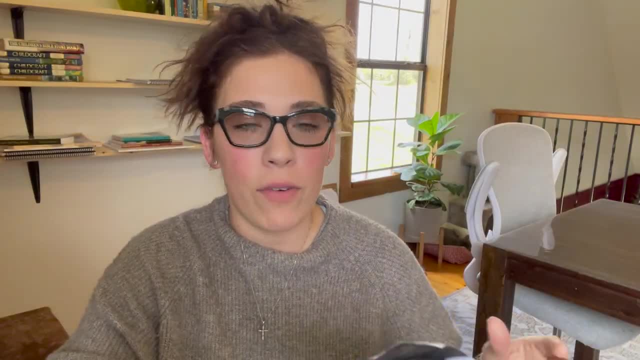 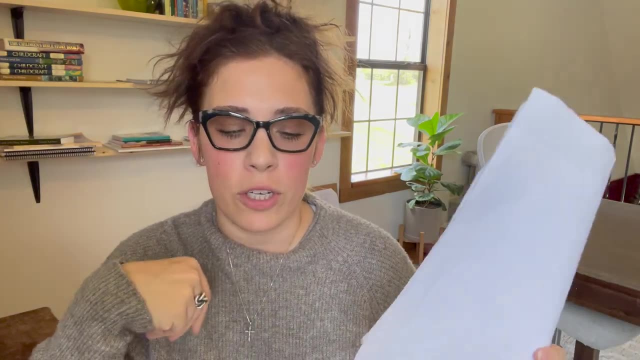 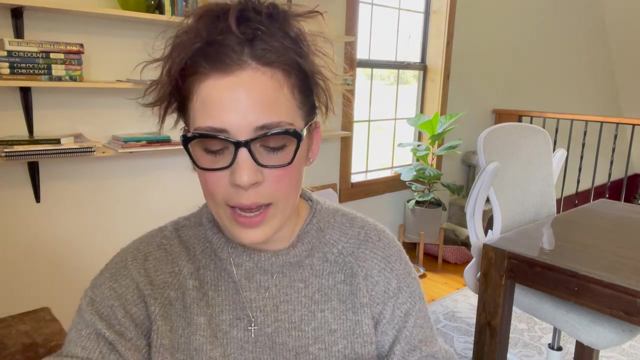 it together and just have that available for every student that's going to be here in the in your classroom setting to recite these every day and just make sure that that's front and center. the other thing, too, is there is a mentioning of what order of operations the 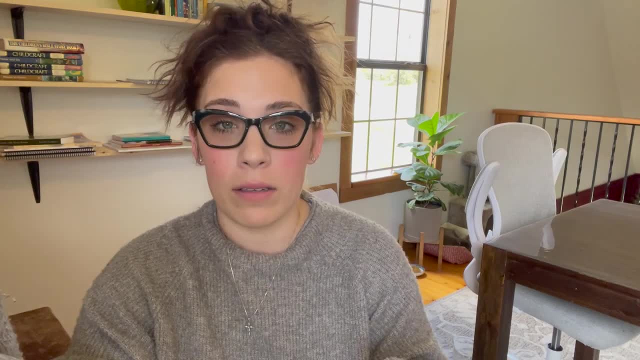 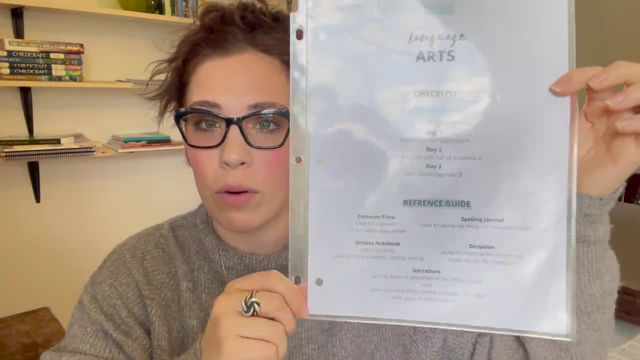 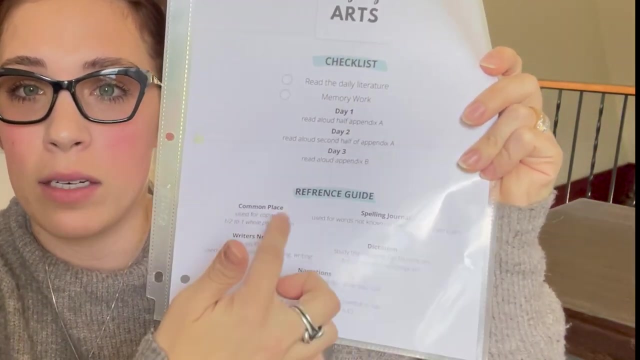 student should do in the very beginning of their their lesson plan book that you buy. I went ahead and typed out for him what he needed to do on each day, as well as a reference guide for what each thing meant when they were discussing it in the book. so the checklist. 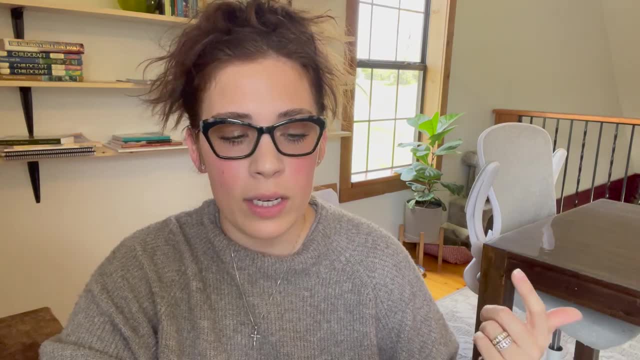 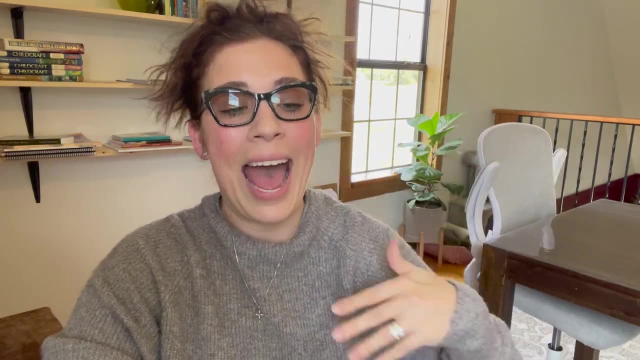 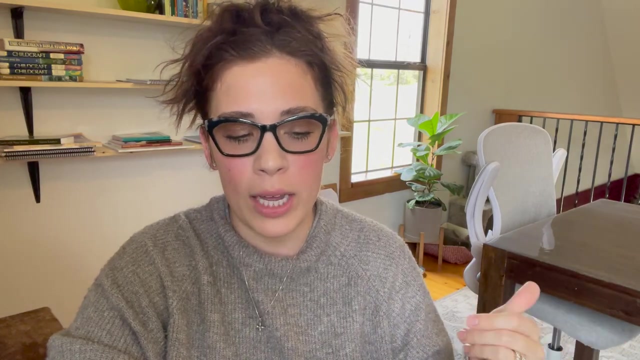 read the daily literature, and he really only needed to use this for maybe the first month or two, because once he got into the the habit of using this new curriculum, it was smooth sailing for him. so the checklist is: read the daily literature and then memory work. so day one. 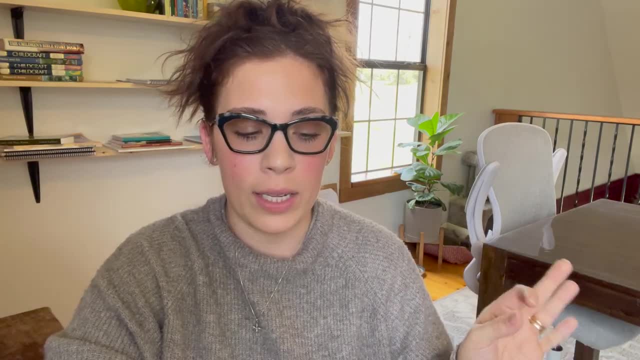 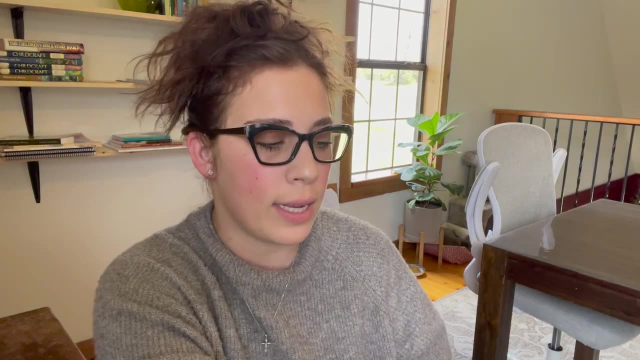 day two, day three, day one I had him doing read aloud half appendix a day two, read aloud second half, and you kind of get what I'm saying and that was just me pulling from what the book already said and then the reference guide. I just wrote down what the commonplace book was, what he was.